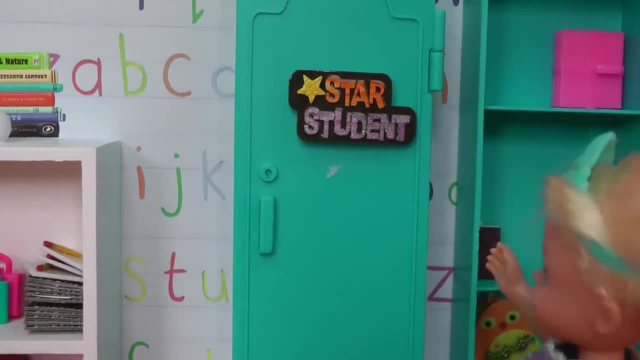 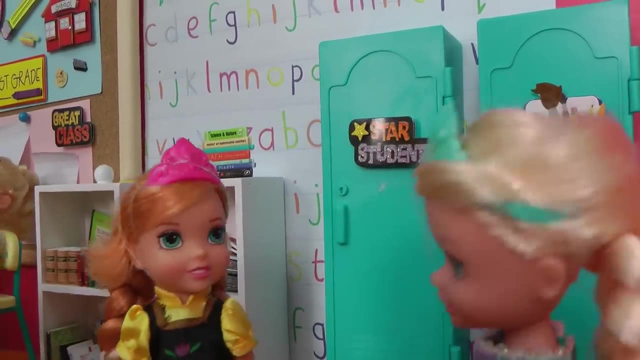 Let me get my book. Ooh, I'm the star student. Wait for me, Elsia. Are you sure he won't bully me? Come on, just follow me. Oops, we're the last ones. Come on, hurry. 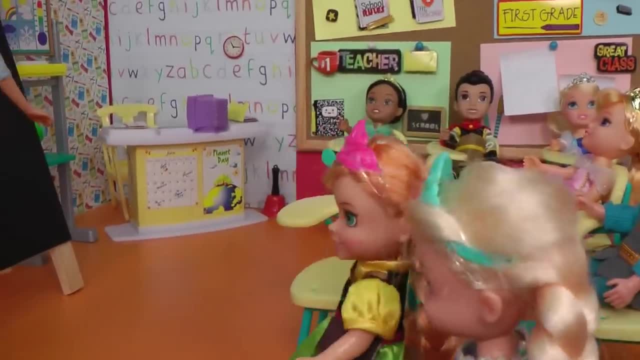 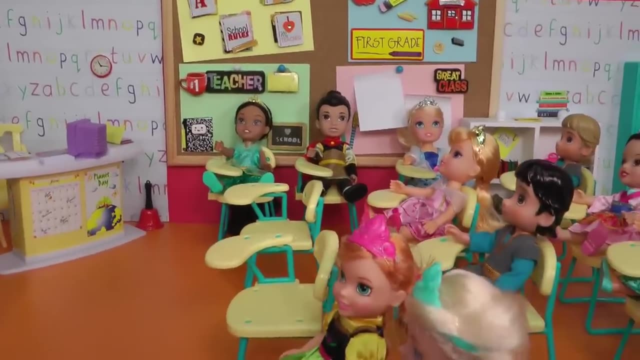 Elsia, Okay, Hi girls. Hi, Ms Natalie, Hi, Well, you're almost late, so you better get in your seats quick. Alright, Okay, time to take the attendance. Just stay here, Anya Here. 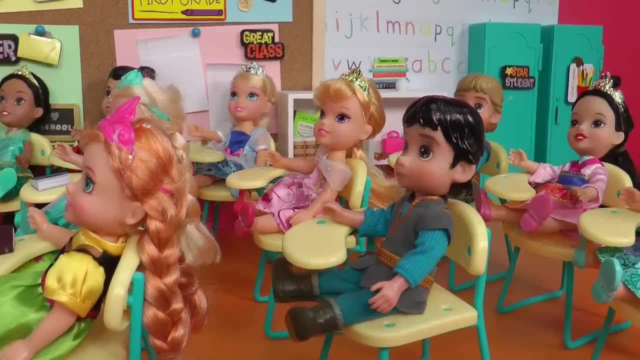 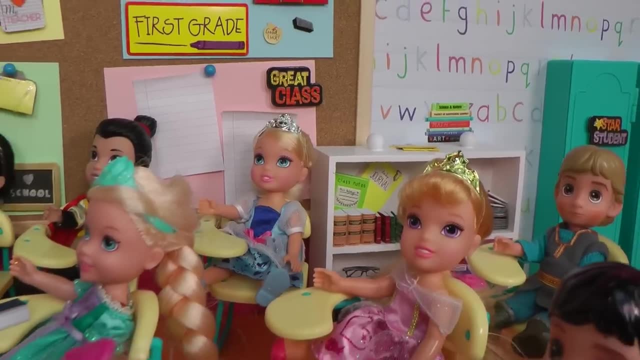 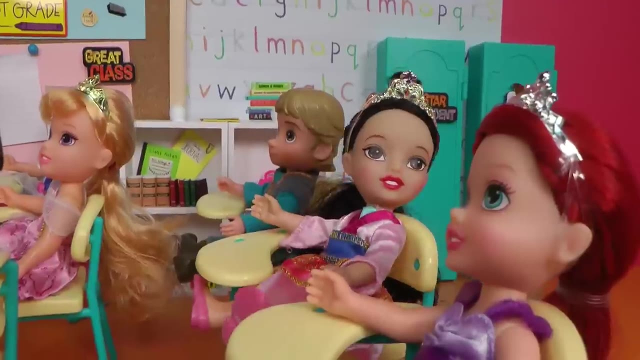 Benjamin, Of course I'm here. I'm always here. Ariella Here, Jasmine Here, Aurora Right here. Cinderella Present, Daniel Here. Two more people, Mulan. Oh I love your dress, Mulan, are you here today? Is somebody sleeping? 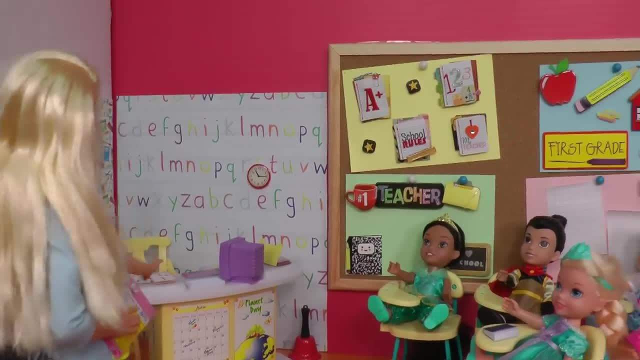 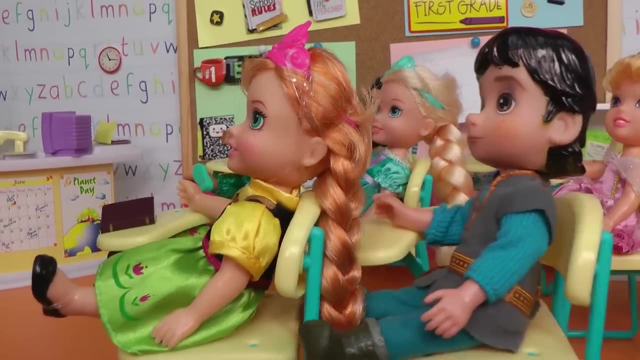 Oh, sorry, I'm here. And last person, Shang, are you here? I'm here, teacher, I'm gonna push Anya. I don't like her at all. Push, push, push. Who's doing that? Hey, you dropped my book. 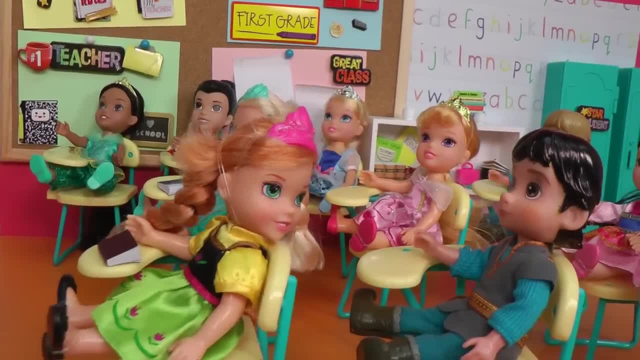 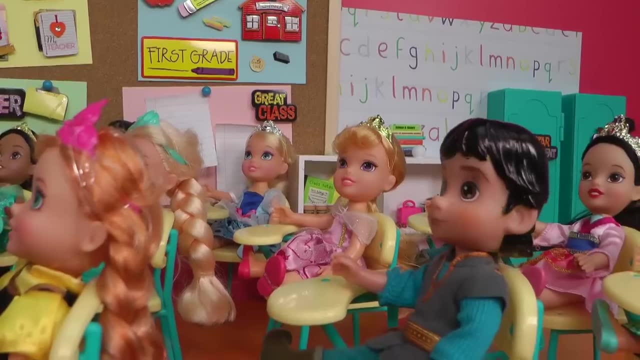 So what? That's very funny. Stop, Or else I'm gonna tell the teacher. Hey, what's going on there? Benjamin, Please be nice to Anya Chicken. It's time to sing the ABCs. I like them. 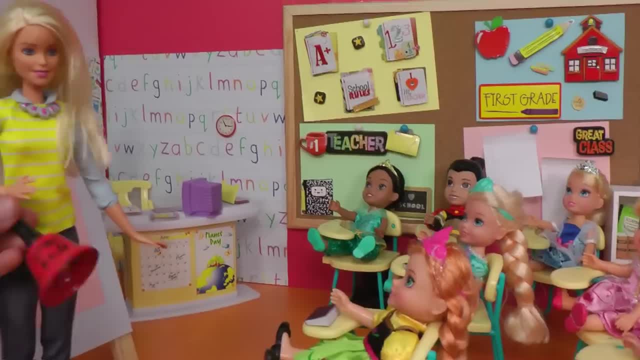 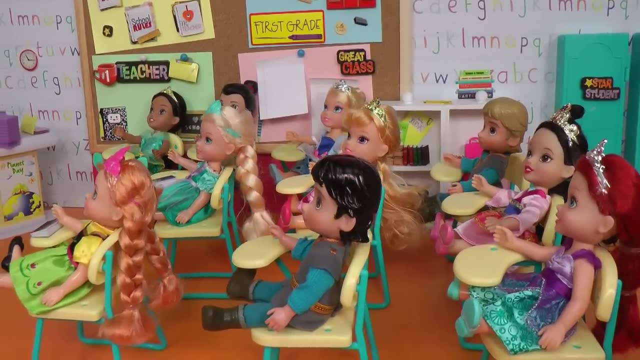 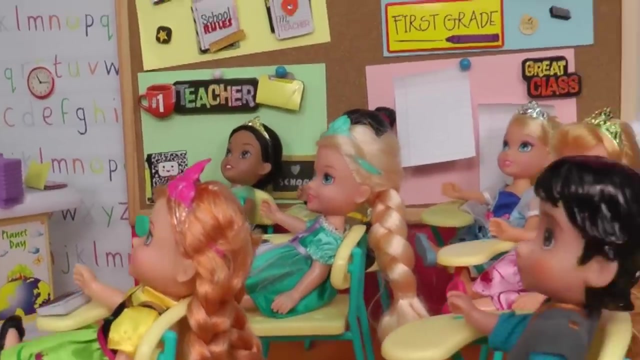 Class. why are we talking? Everybody listen Quiet. Is everybody quiet now? I don't want to Everybody. do you want me to ring it even louder? No, okay, We will stop. Okay, it's time to sing the alphabet. 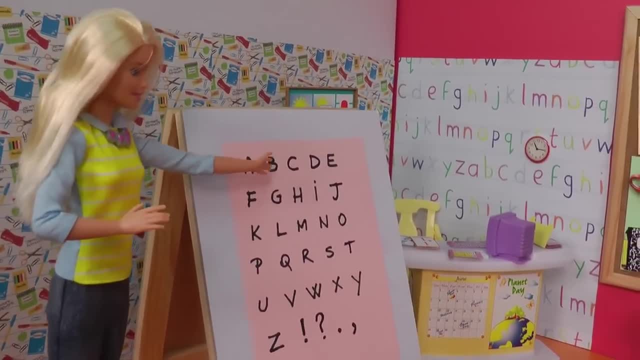 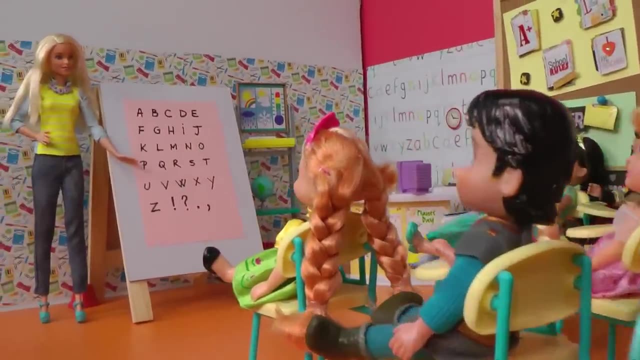 Three, two, one go A, B, C, D, E, F, G, H, I, J, K, L, M, N, O, P, Q, R, S, T U V. 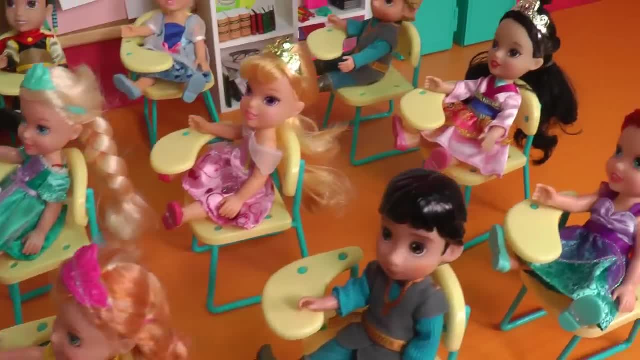 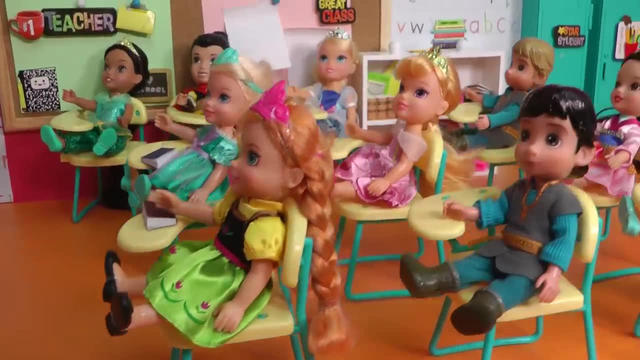 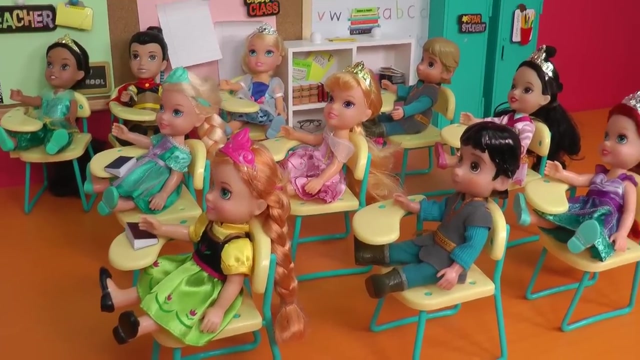 W, X, Y and Z. Now we know our ABCs. Next time, won't you sing with me? Great job everybody. That was so awesome. Thank you. Yeah, that was way too easy for me. For Anya, it's so hard. 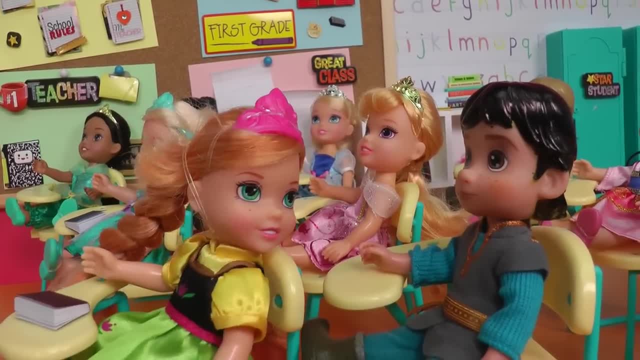 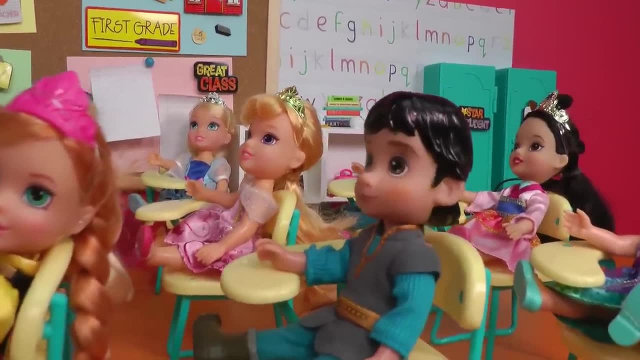 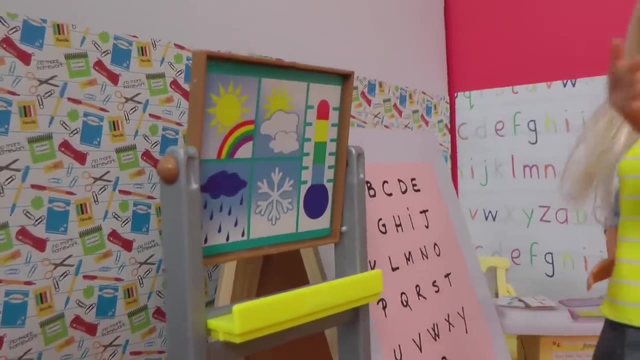 Stop, And I'm getting really mad at you now, so please just stop it. Oh, what else Your mommy is going to save you And plus, I will not talk to you anymore. Hey kids, who can tell me what the weather is like today? 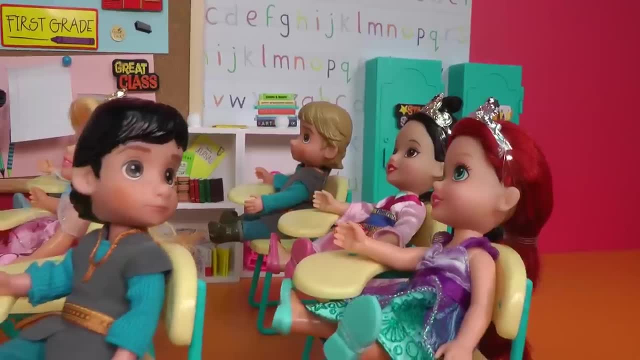 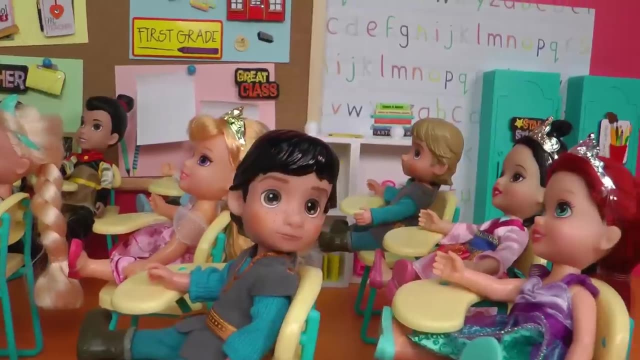 So simple. I'm not even going to bother to do this. Do you think you are the smartest guy in the world? Of course, Ariella. What else I'm so smart? Well, I don't think so. Hey, you stop that, Okay. 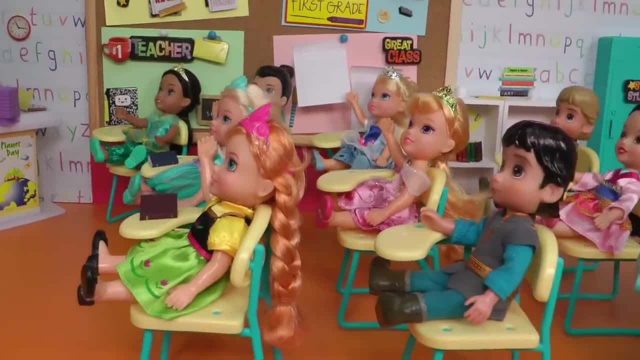 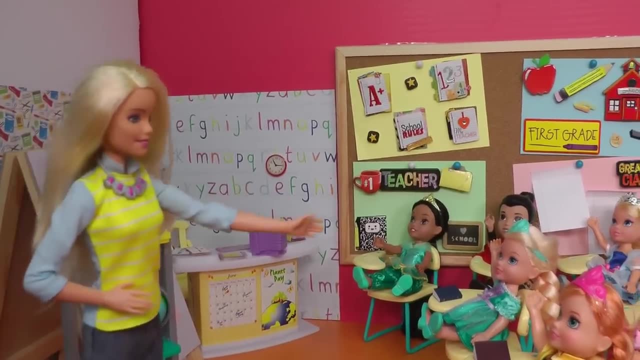 Boy, he's a real bully. Me, me, me, me, pick me, please, please, Okay, whoever is the quietest, I will choose them. Okay, Anya, you can tell me? Okay, um, the weather is. 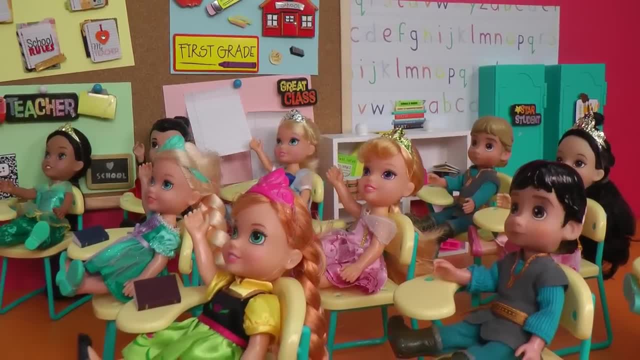 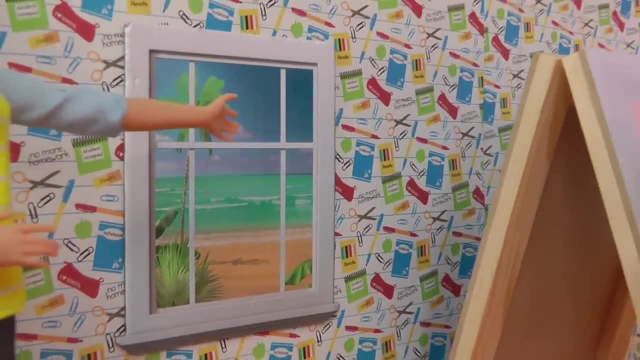 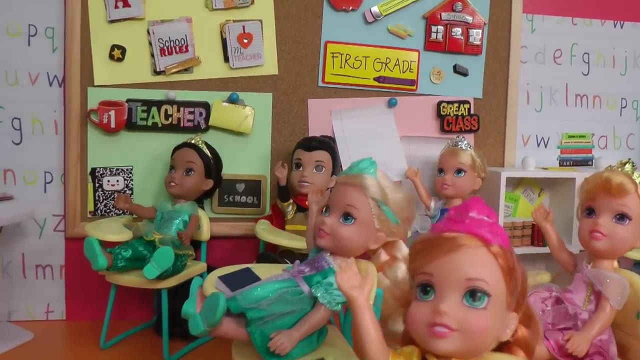 raining, right? No, Anya, that's not correct. Look outside the window over here. It's not raining. I don't. I don't know what it is. Okay, does somebody else want to tell me the answer? Oh, me, me, me. Okay, Elsia, what's the weather outside? 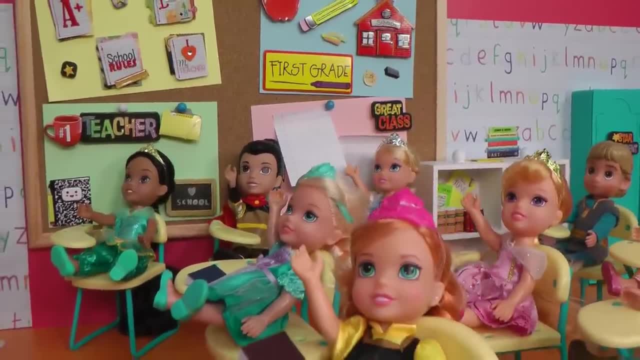 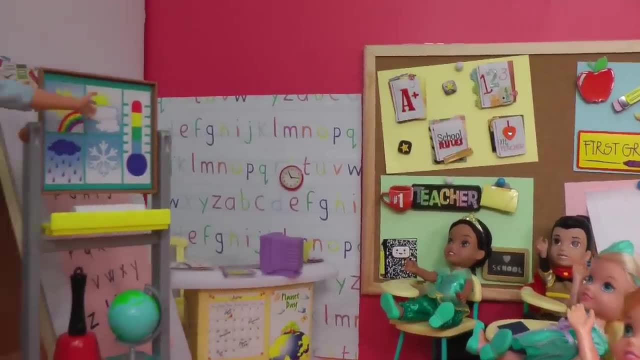 The weather is sunny, Correct, See, Anya, it's not raining, It's sunny outside, okay, Oh, okay, See. so which picture is it? This one, this one, this or that? It's the first one, Yes, and it shows a rainbow, because it's. 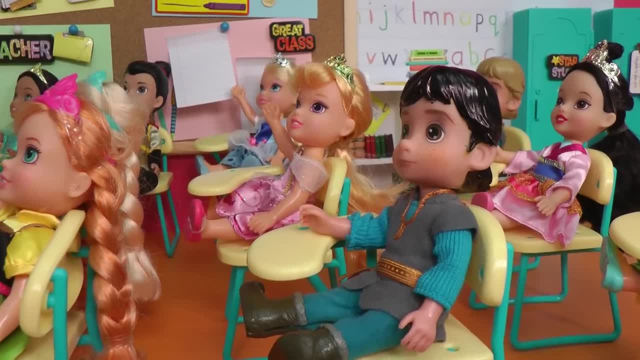 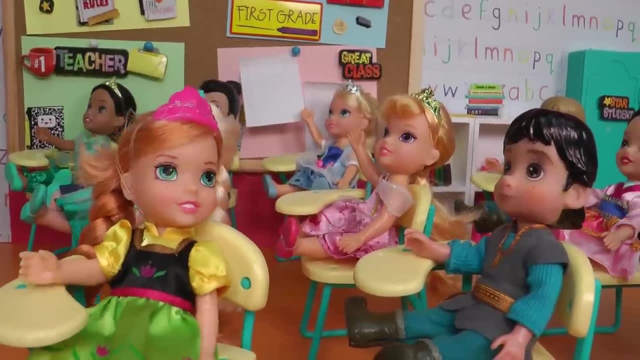 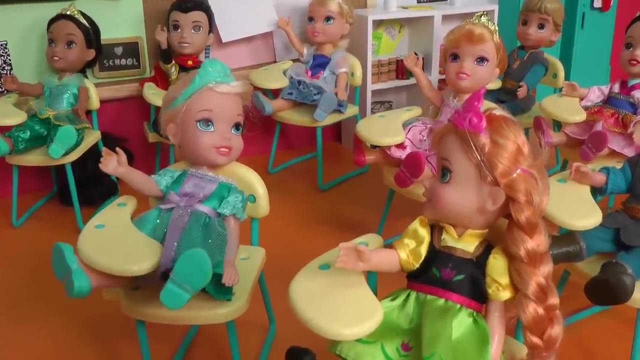 super sunny outside. Wow, Anya, you're so silly. How is that hard? You just have to look out the window. I made a mistake, and so what? And why am I even talking to you? Chicken, Anya, I see what he's doing to you, and if he does it, one, one more time. 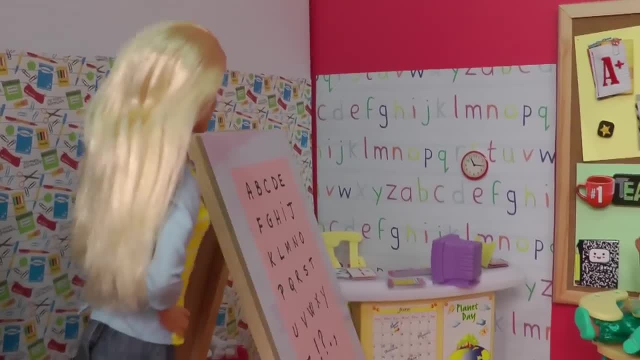 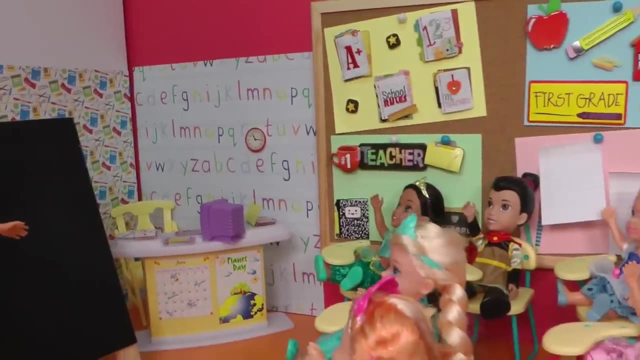 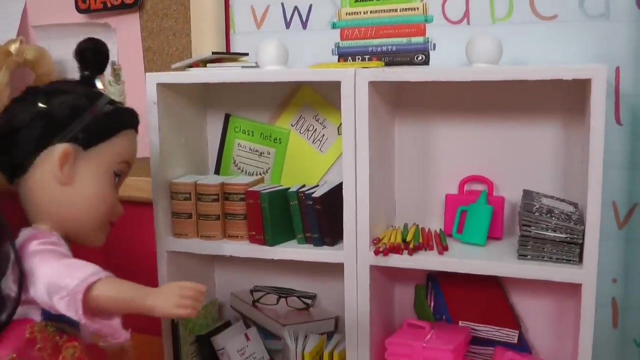 let's, let's tell on him. okay, Now it's math time. math time. Everybody get notebooks and pencils. Who would like to bring them? I can bring the notebooks And I'll bring pencils for everybody. Is it there? Oh, there they are. 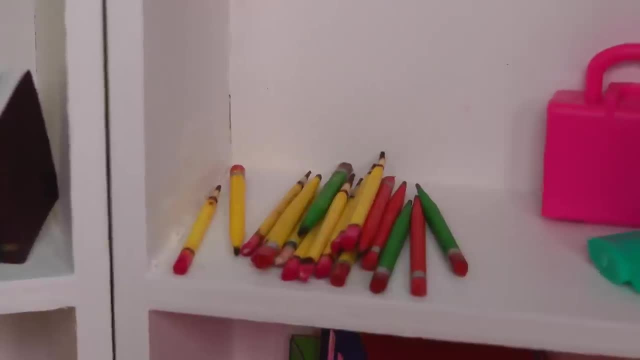 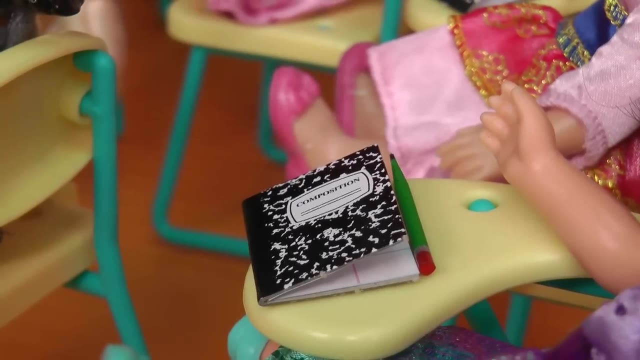 Get the notebooks. There are the pencils: One, two, three, four, five, six, seven, eight, nine, ten Enough for everybody. Does everybody have a notebook and a pencil out? Yes, No, no, I don't. 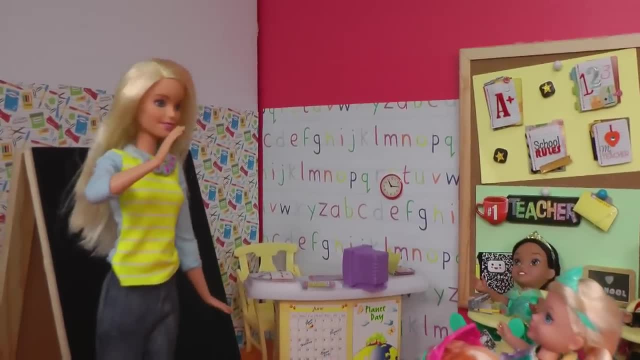 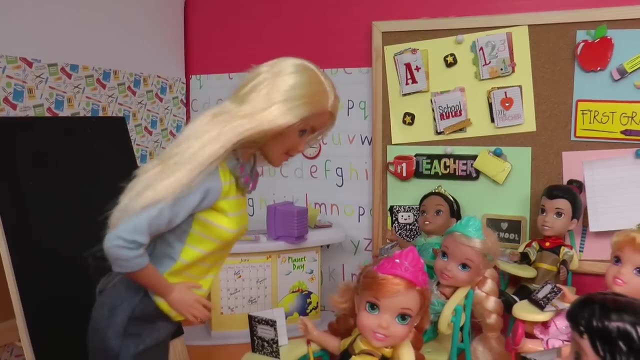 What do you mean, Benjamin? I see a pencil on the desk there. Well, I do have a pencil, but ew, it's ugly. I want another one right now. teacher Benjamin, you have to start learning to be nice. I don't like your attitude. If you want another, 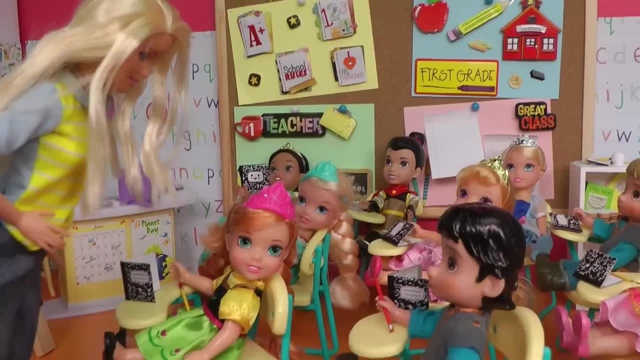 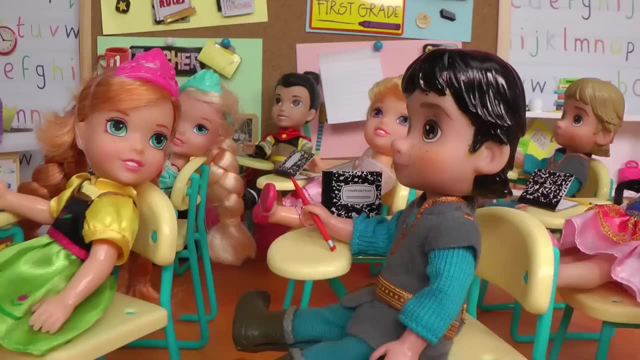 color. just tell me, nicely, You don't have to be rude. Okay, fine, sorry, Can I please have another color? See, that's how it feels. Oh please, Anya, mind your own business, Don't care about me, I'm the best anyway. 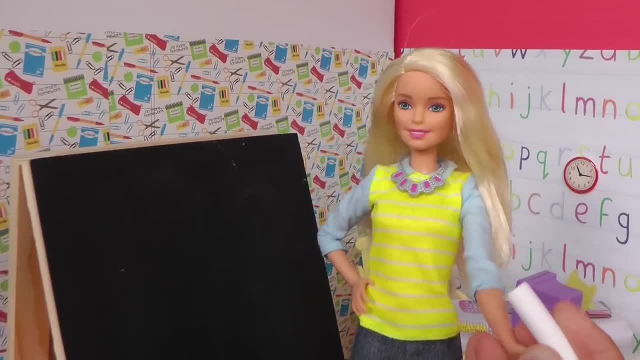 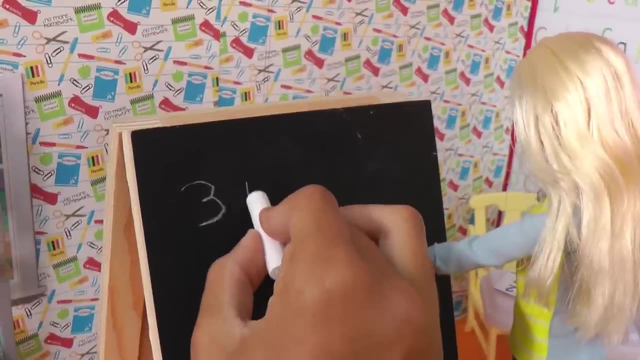 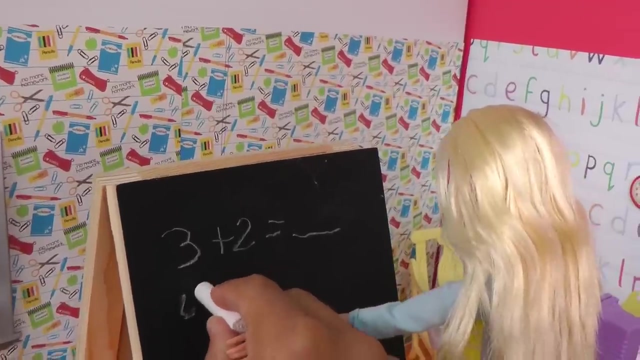 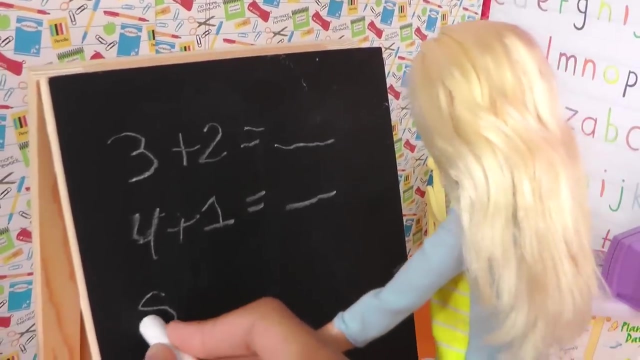 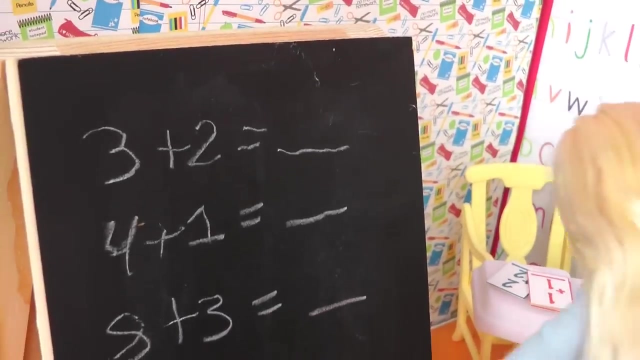 Yeah right, bullies. Okay, hush children, We're learning math. now I'm going to write some problems here. Three plus two: the answer. How about? four plus one? eight plus three and two more: How about? 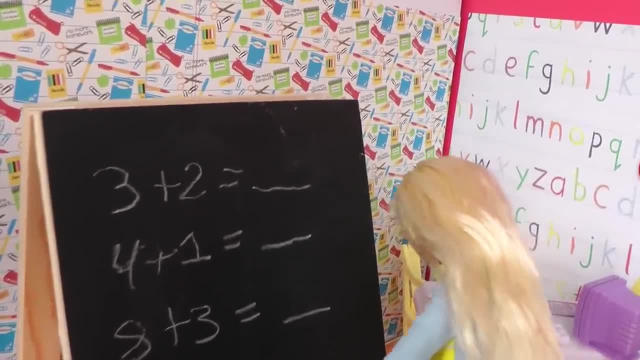 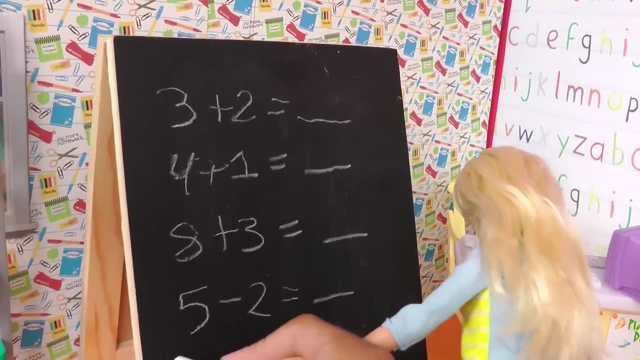 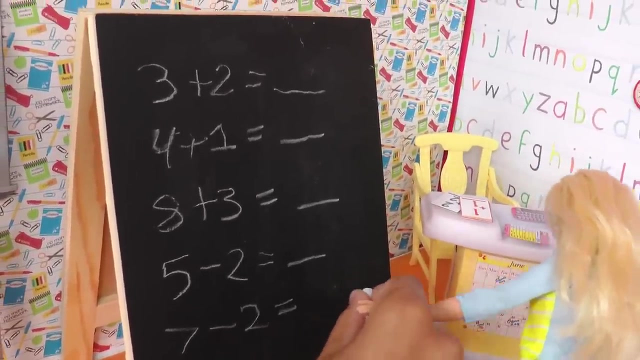 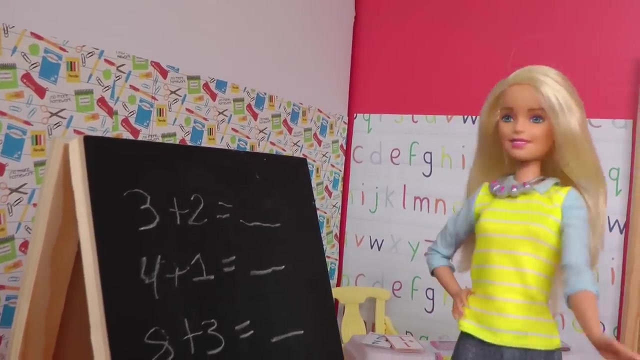 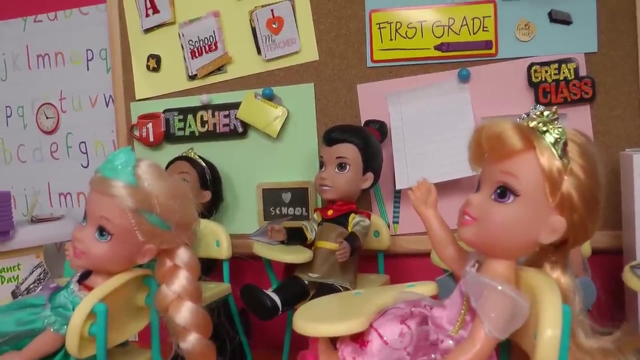 five. let's do subtraction. Five minus two and seven minus two. Okay, who wants to do the first question? It's three plus two. Who knows the answer? Can I say the answer please? Of course, Aurora. What's the answer? Um, the answer is. 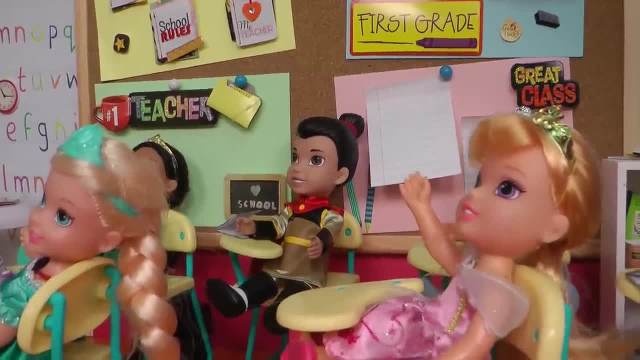 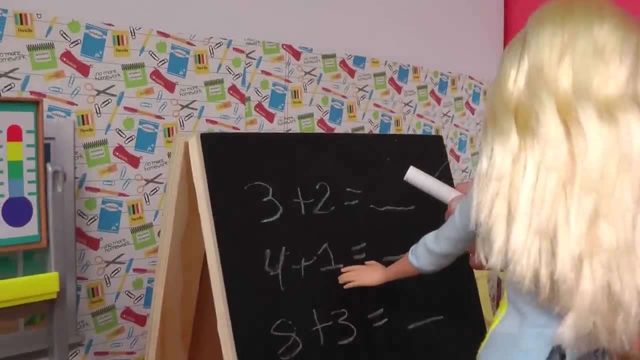 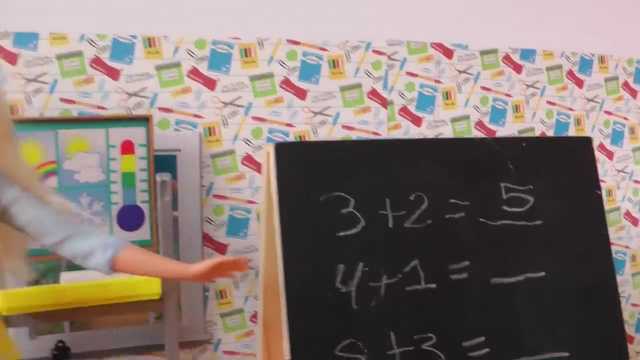 five. Yes, that's correct. Yay, I got it right. Okay, I'm going to write it on my board. So three plus two is five. Good job, Yay, thank you, teacher. Okay, let's see who can answer Four plus one. 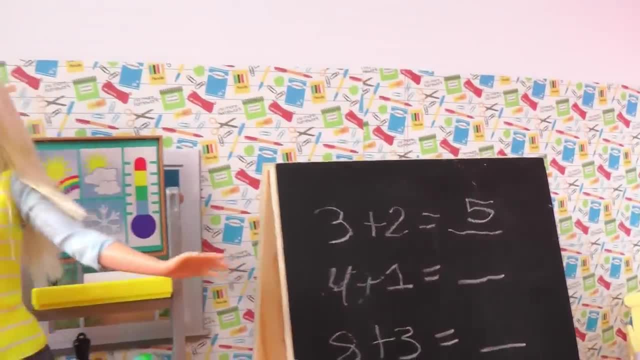 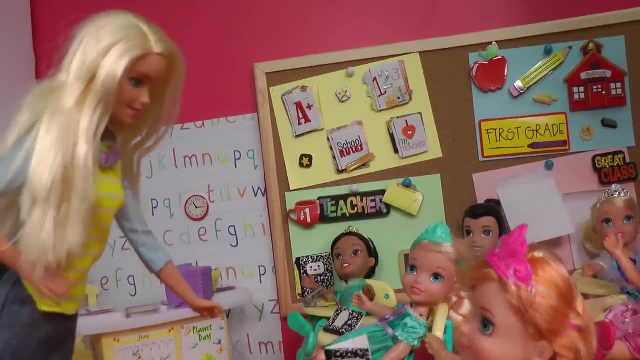 Hmm, nobody wants to answer, then I'll choose Anya. you answer this, please. Oh, um me. Yes, you Come on, Anya. you know the answer, don't you? Well, I'm still thinking, Anya, do you even? 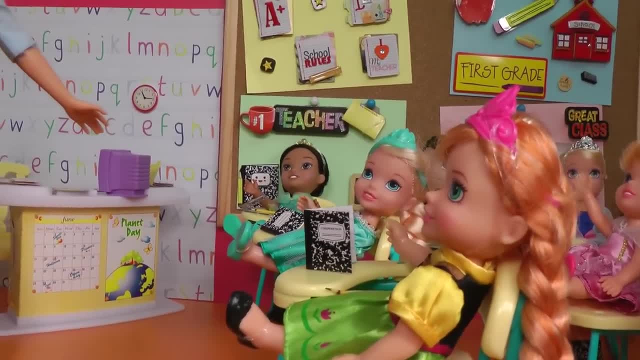 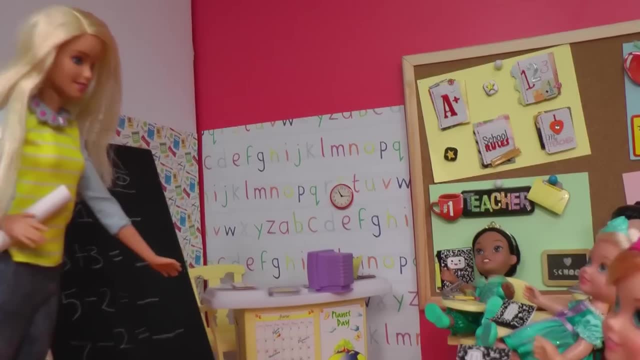 practice math at home. Um, maybe, just um, I don't know. Oh, Anya, I'll help you. Come to the board. I'm waiting, Anya, why are you not coming? I told you to come. Um, maybe tomorrow, not now, okay. 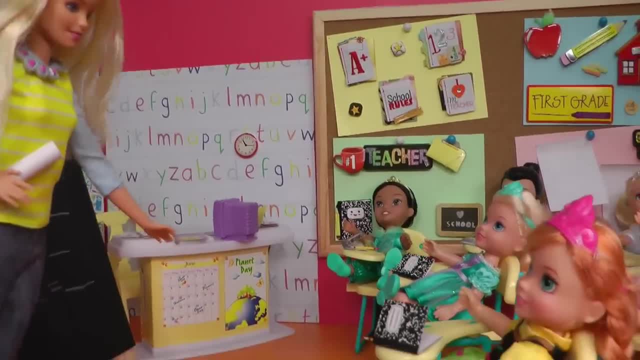 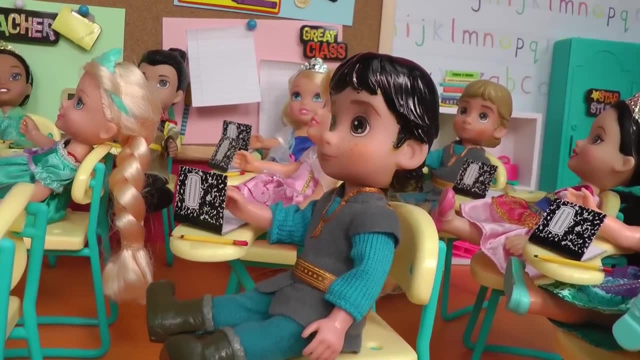 Anya, don't be silly. I told you right now, Out of your seat, please, No, but but please, Anya. last chance. Okay, Anya's afraid and doesn't want to go because she doesn't know the answer. Go, Anya. 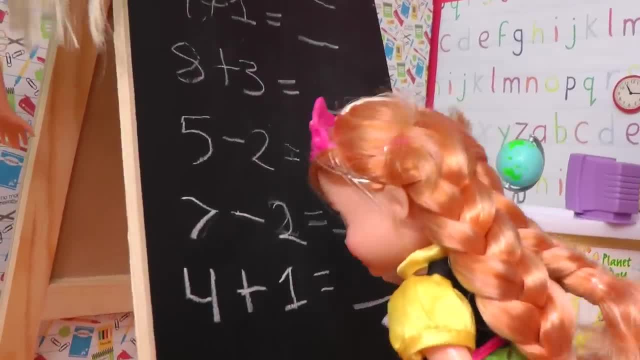 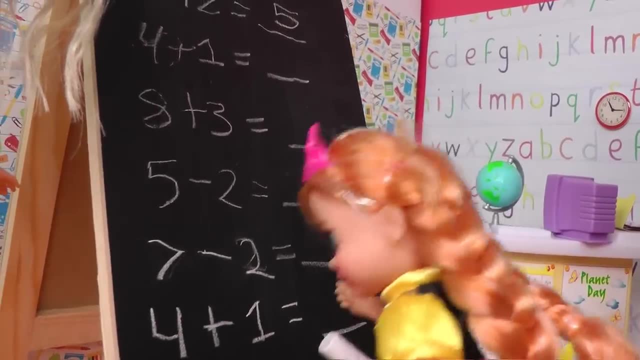 tell me the answer. So what's the answer, Anya? Okay, so four plus one. I don't know I, you know I can't, No, I can't. I don't care about the four, so it's one. It has to be ten, Put a one. 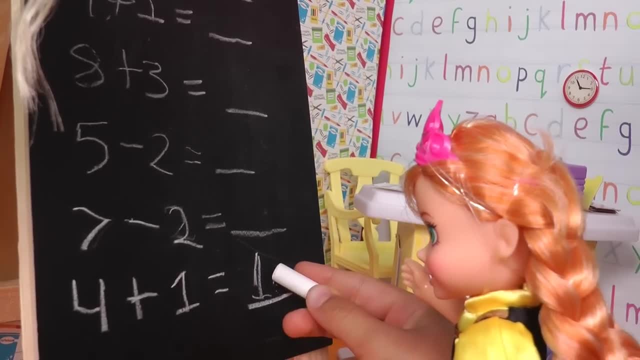 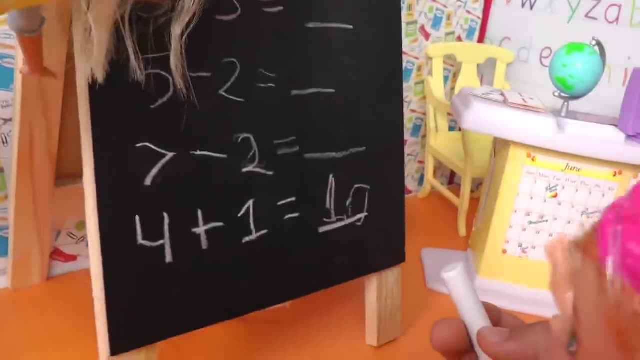 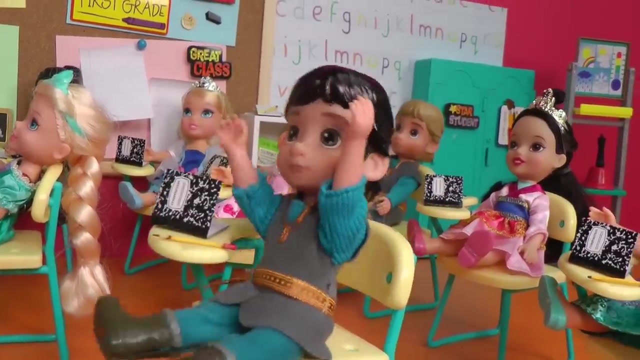 down there and a zero. Let me see What's the answer. It's ten, right, Anya? how can four plus one be all the way to ten Ten? eh? A? sia said four plus one is ten. Did you hear that, guys? 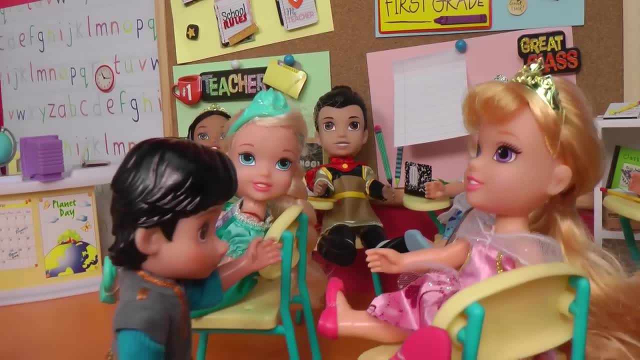 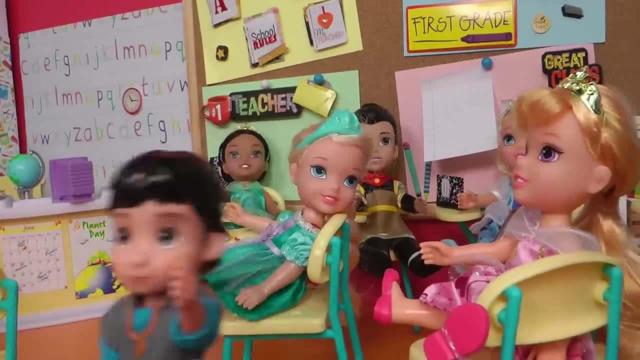 Hey Benjamin, that's not nice. She just didn't practice, She'll learn. Yeah, who's talking here? Come on everybody. Anya doesn't know anything. Anya doesn't know anything. We're not going to say that. 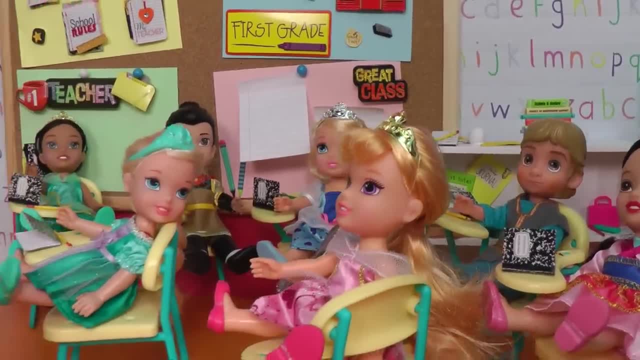 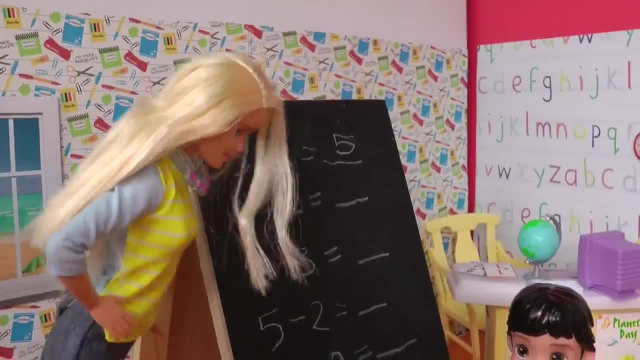 That's rude, Very rude, very rude. Anya doesn't know, know anything. Anya doesn't know anything, you don't know anything, Anya. hey, let me show you how I do one, Benjamin, remember I don't like your attitude and you're. 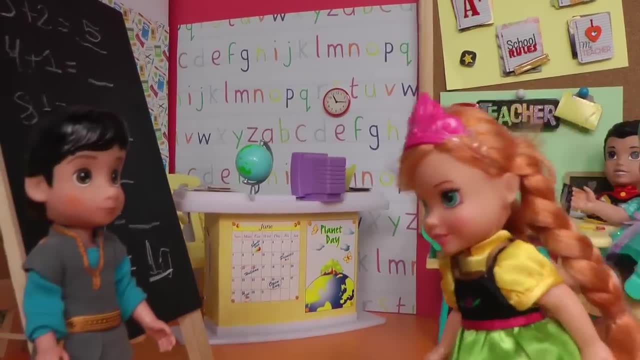 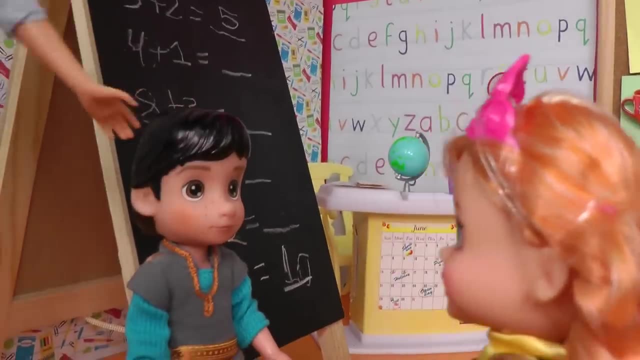 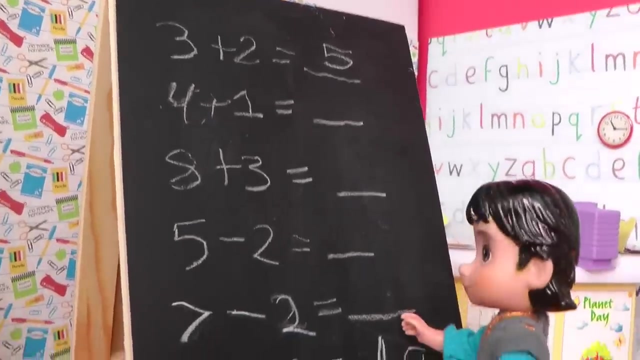 not being nice to Anya. hey, I told you to mind your business. that was rude. I was trying my best. actually, Anya, why don't you take a seat and let's see if Benjamin can do the rest of the questions? oh okay, see all these questions, I will answer all of them, right? so let me just take this silly. 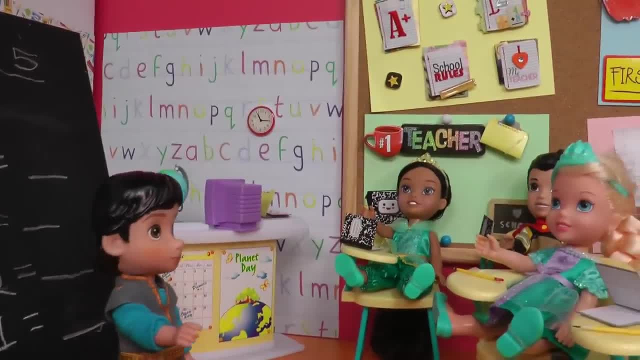 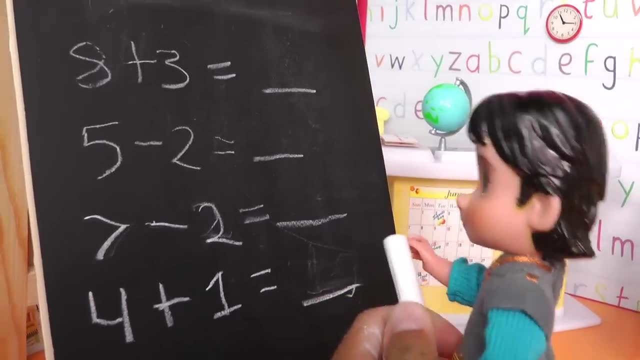 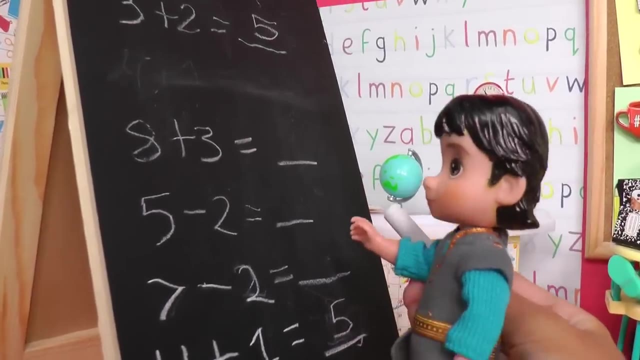 answer out ready. everybody watch me the awesomeness, sure? whatever, four plus one. I don't even need to draw any dots for this answer. Wow, Anya, it's only five, not ten. seven minus two. hmm, this is also five, so easy. I want to go to grade two. 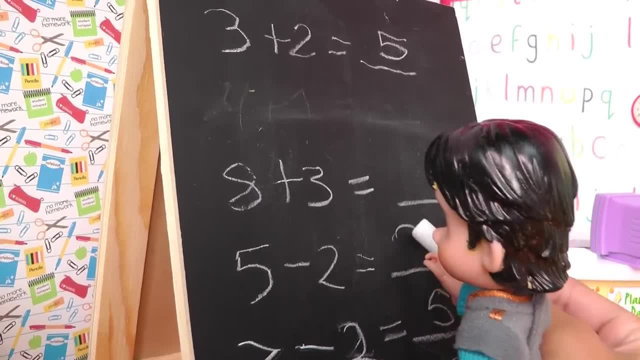 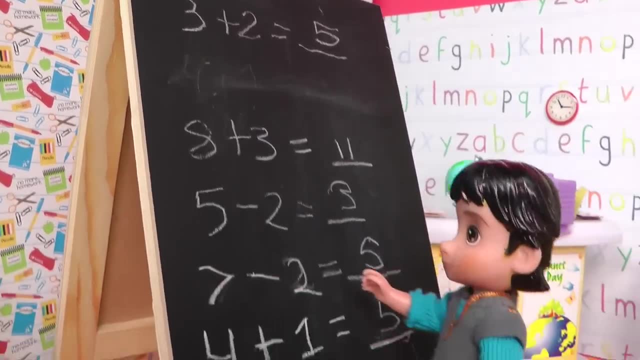 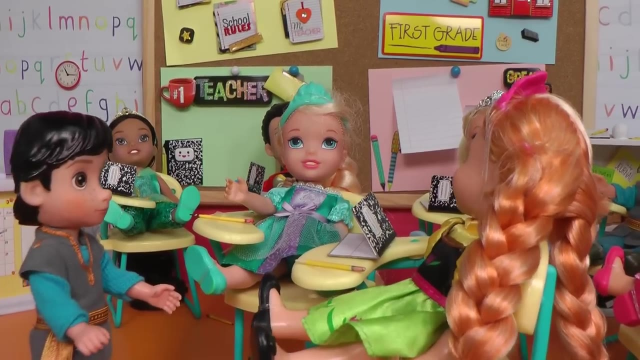 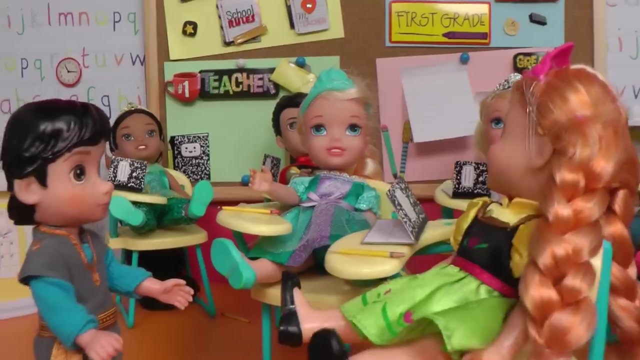 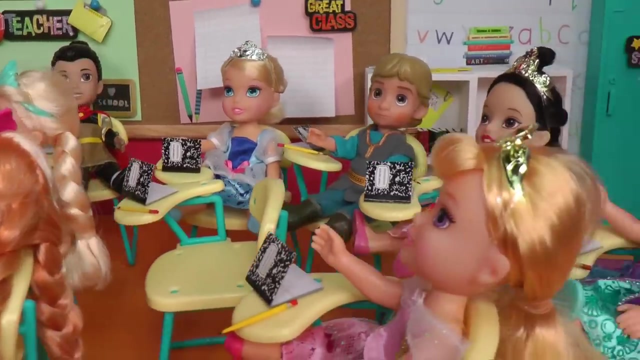 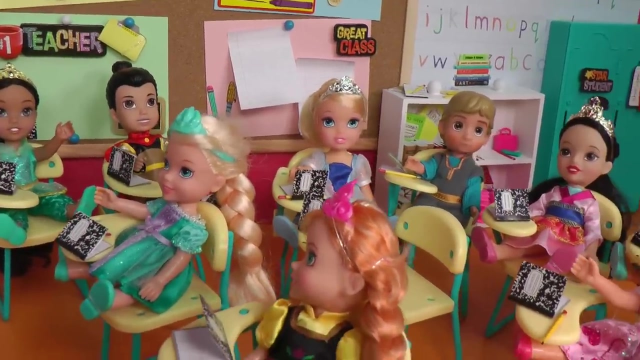 five minus three, wow, this is three, and eight plus three is eleven. I know all the answers, see. oh, yeah, I'm the best. yes, I'm the best. ha, did you hear that guy? she wants her mommy cuz I'm too good, don't you agree, guys? oh, stopped, yeah, stop it. we don't have it, yeah, stop it. Benjamin, yeah, that's it. 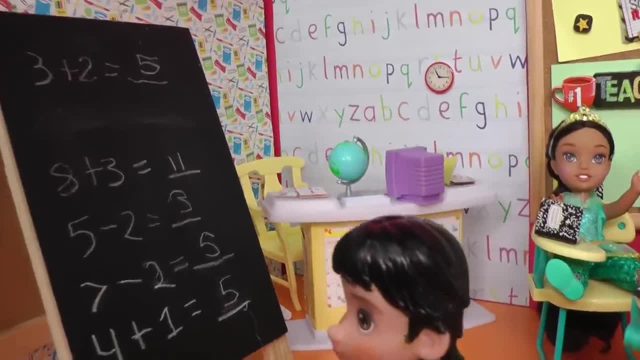 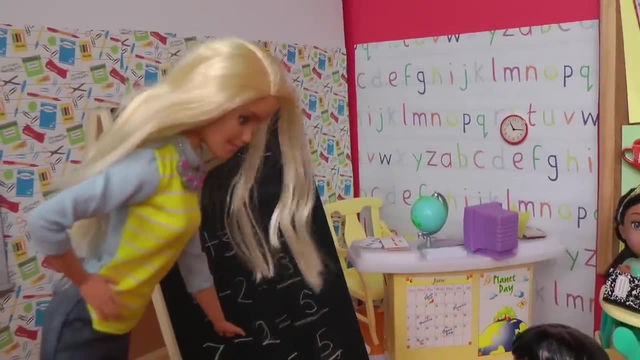 Benjamin, I have good and bad news. the good news is that you got all of the questions right. oh yes, I knew I was the best shh stop. you are rooted. I don't like your attitude and I told you too many times. that's the bad news going. 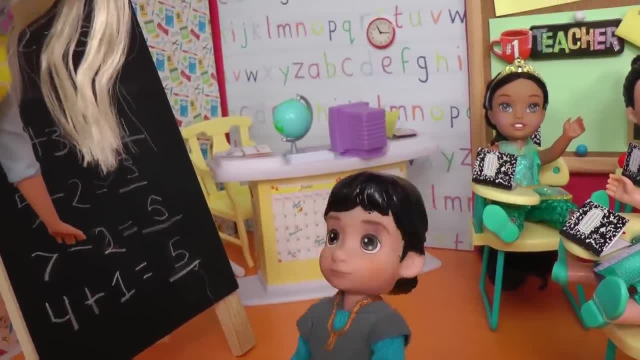 timeout, and I'm gonna tell your parents about this too. no, no, no, don't do that, please. sorry, I have to do it and you may not be good to me. no, no, no, don't do that please. sorry, I have to do it and you may not be good to me. 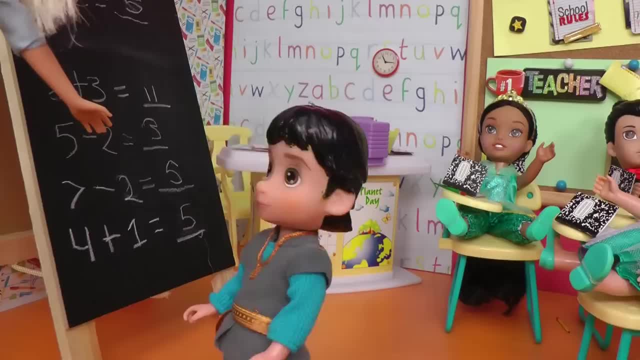 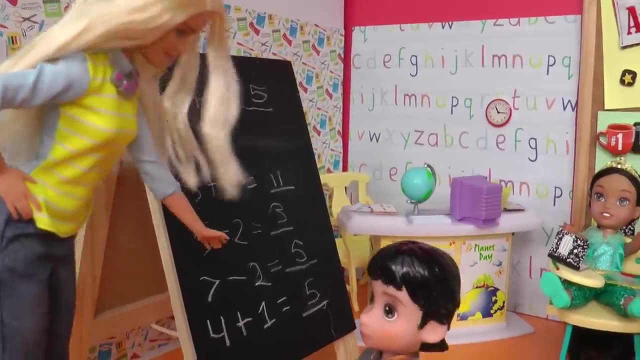 made Anya cry and I don't like this in my classroom. Fine, I'm sorry, teacher. Everybody should know that this is not acceptable in our school or classroom. Understand? Yes, I understand, I'll go out. Uh, sorry everybody. 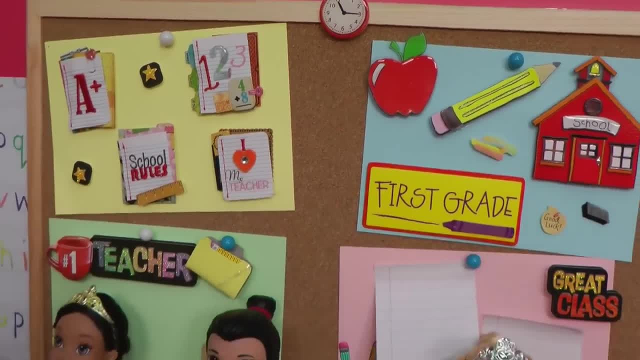 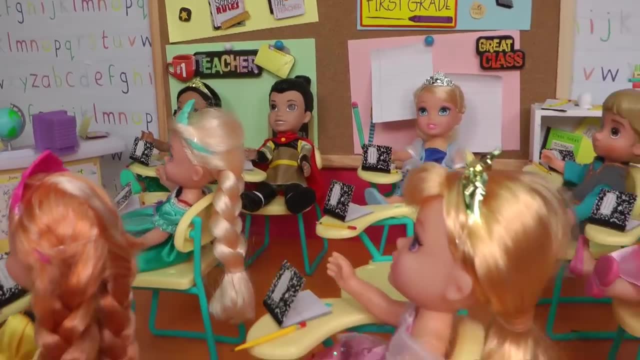 Yay, It's time to go home. Yes, that's right. I'm sorry, but that's all for today, so pack your bags and you can go home now. Yay, Bye-bye, Bye, children, See you tomorrow.